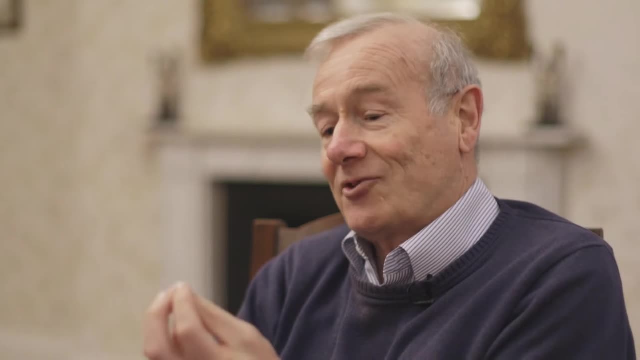 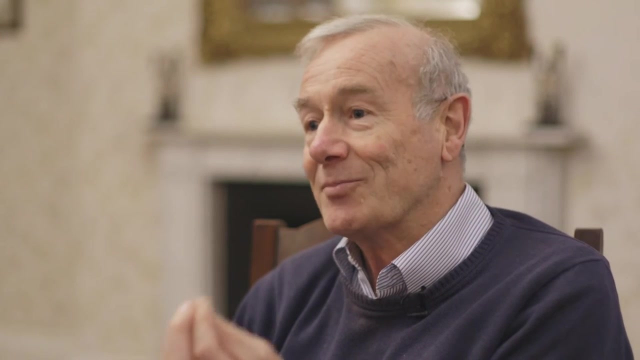 protons and neutrons when they touch, And that's what holds the nucleus together. So the neutral neutrons add a much stronger force to the nucleus than electrons, And all of which don't feel the electrical disruption, are very important in helping nuclei stabilise. 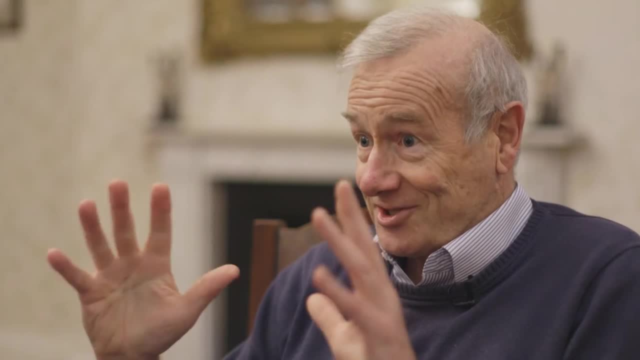 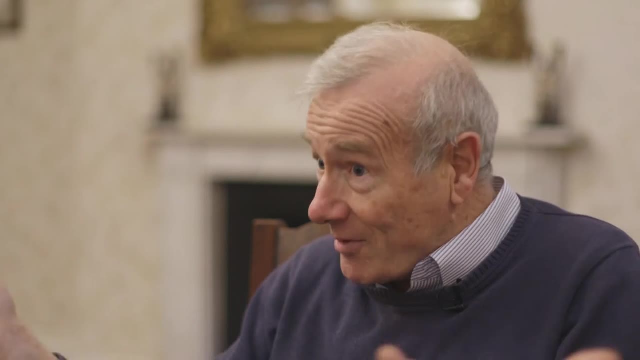 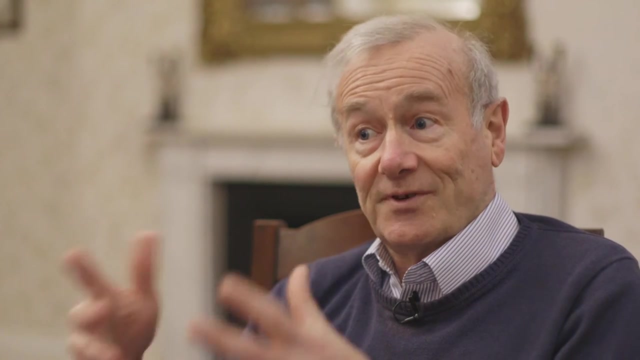 Number six: radioactivity. Not all nuclei are stable, Some decay and change form, emitting radiation in the form of alpha, beta and gamma rays. Number seven: perhaps the most famous unstable nucleus is the case of uranium and the property called fission. 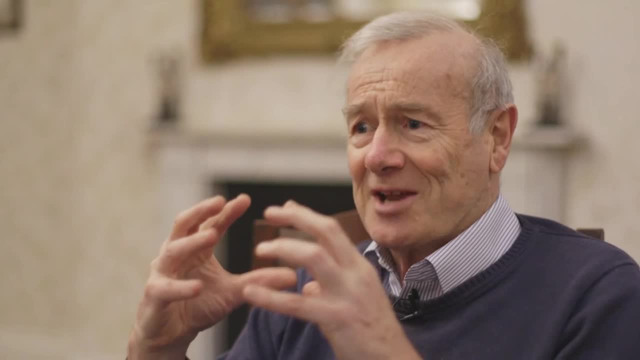 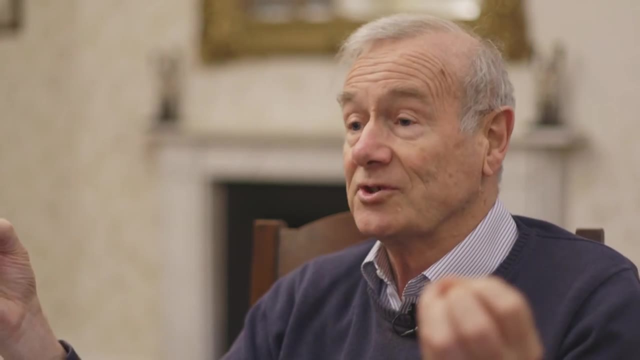 Uranium has got so many protons it's only just able to hold together and the slightest nudge like a single passing neutron can split it into two. That's what we call fission, And that releases energy- thousands of times as much energy as you get in an ordinary chemical reaction. 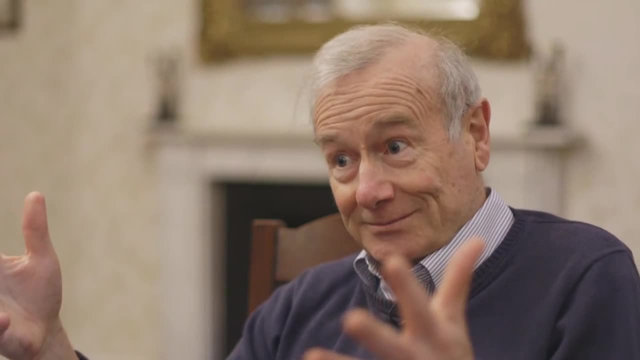 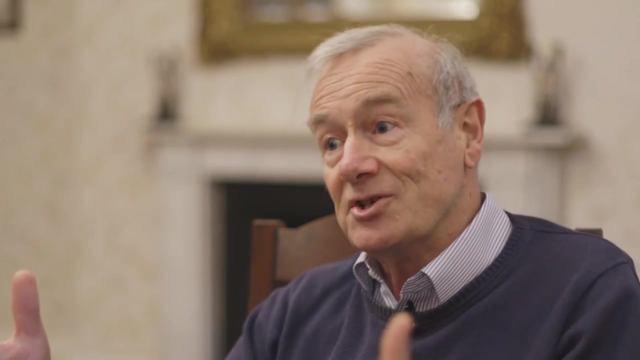 Number eight. we had fission. now we have fusion At the other end of the periodic table, where hydrogen lives. light elements, if they join together, can release energy And that's called fusion releasing energy. So, for example, hydrogen. 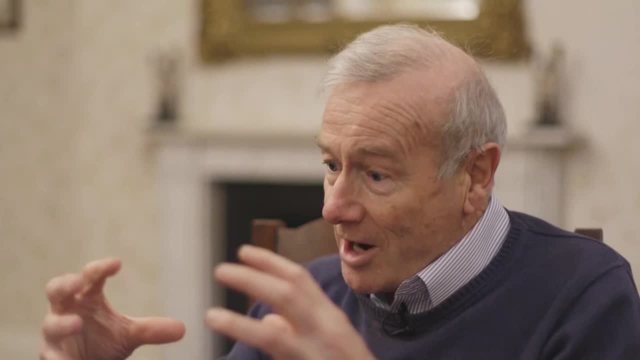 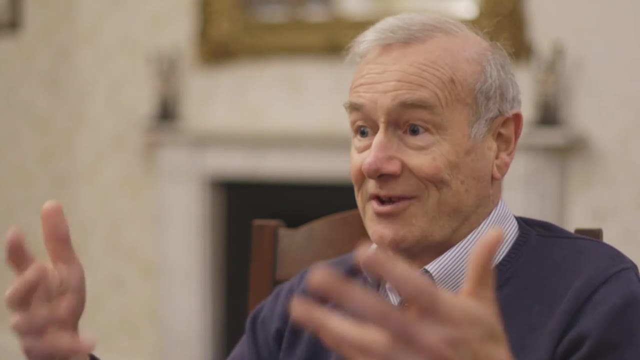 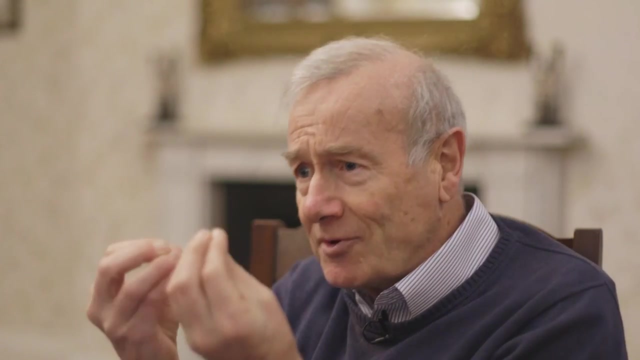 which is the fuel in the sun. when hydrogen joins together, it can turn into helium, the next element in the periodic table, and release some energy which eventually we feel here as sunlight Number nine. one of the miracles of nature is that if three helium nuclei happen to touch, 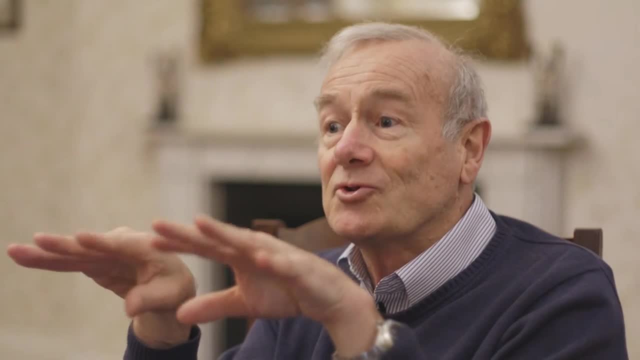 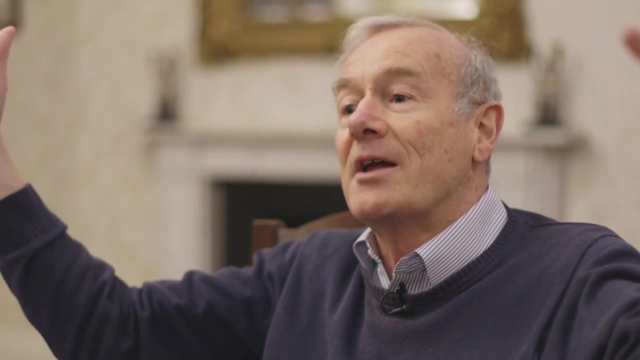 magically, this is exactly the same as what's called a resonance level of carbon, And that is how carbon is made, And in hotter and hotter stars you can build up heavier and heavier elements until eventually, in some cases, the star explodes, called a supernova. 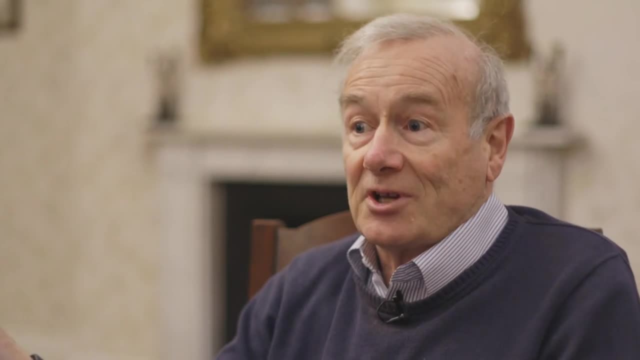 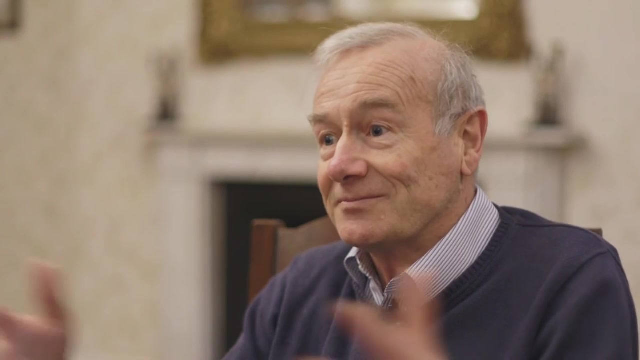 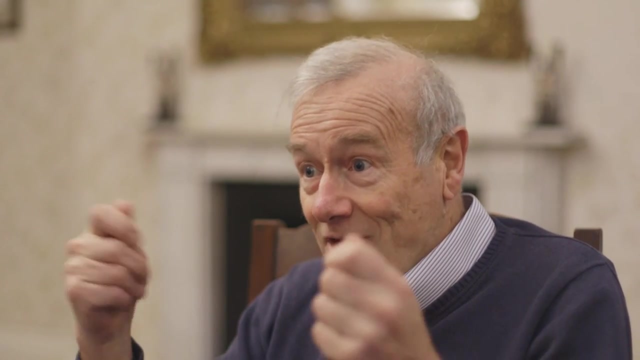 throws all of these elements out into space and eventually they might form the seeds of planets and other stars and people someplace. Number ten is the nucleus. as a detective, The phenomenon of radioactivity gives us a natural chronometer. Like in uranium, it's half-life. 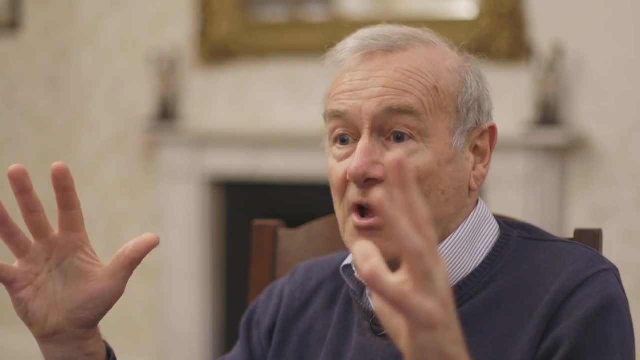 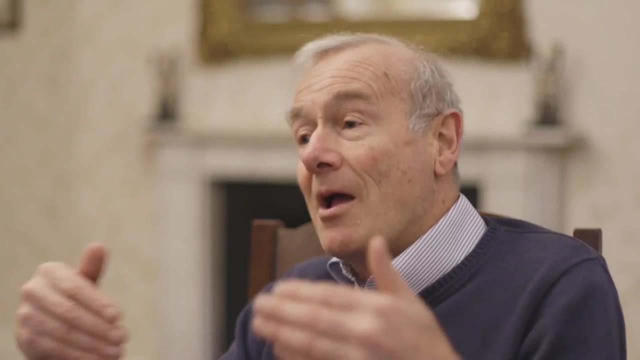 That means, if you have a sample of uranium atoms, half of them will have decayed and half of them will have disappeared, And that's what we need after about five billion years, which is the age of the Earth. pretty well, And so by measuring the abundance of different isotopes of elements like uranium,